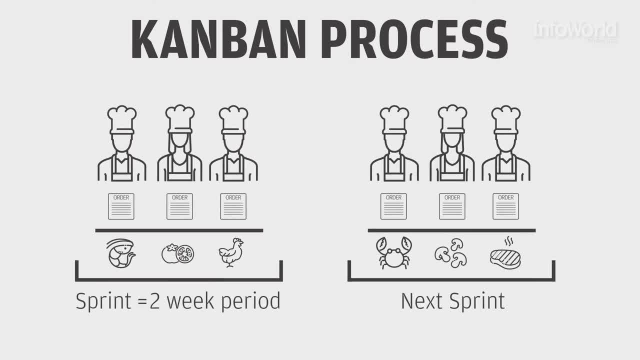 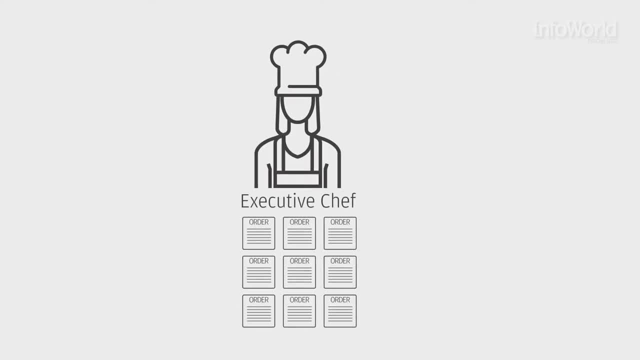 the various developers work on their tickets so they're done in time for the next sprint. In a restaurant, the executive chef shows the cooking team everything that needs to be done for this set of orders. The cooks commit to what dishes they will want to prepare. 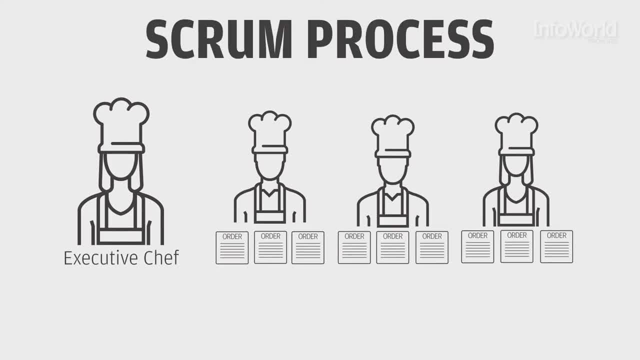 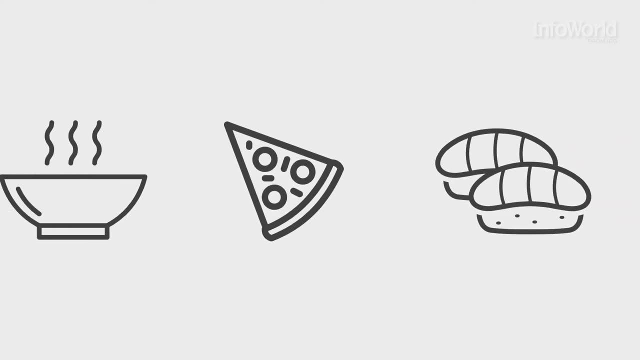 In agile development, the same process occurs in what is called the scrum process. In agile development teams, developers likewise commit for the code. they will deliver for the current sprint. The cooks make the food, adjusting the seasoning and methods as needed based on the ingredients. 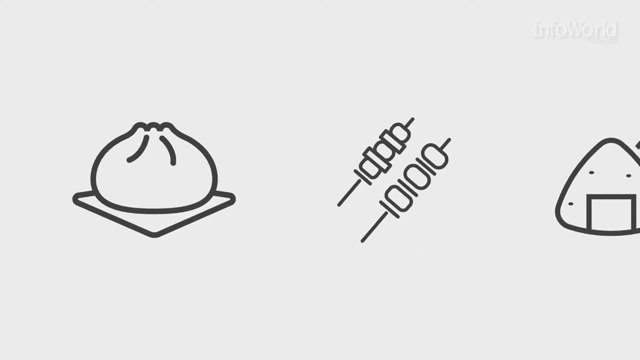 they have and any issues that come up while cooking to deliver the meal the customer expects, as well as from any feedback from the wait staff and customers. Agile development works the same way. Developers implement what they committed to making adjustments as they go to deliver. 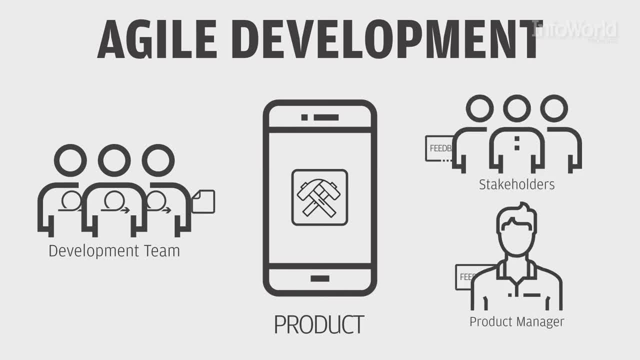 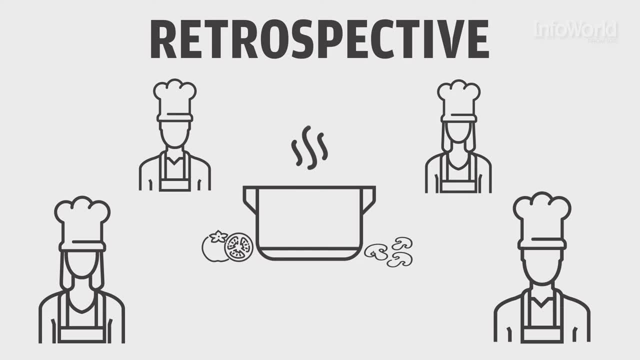 the desired result based on feedback from stakeholders, the product manager and their own insights. A restaurant's cooks are always looking to make the food better and the preparation process better. As they cook, they discuss and record where they need to make improvements with the ingredients or cooking process, then make adjustments in their future work Agile. 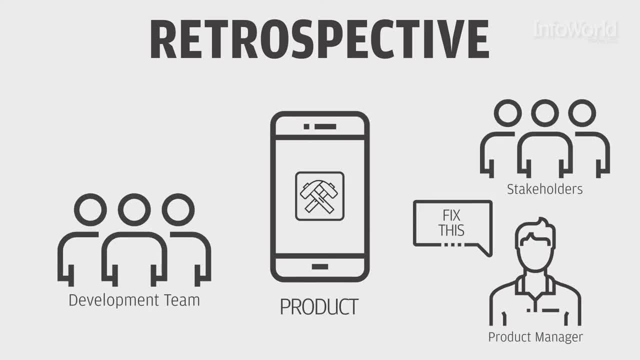 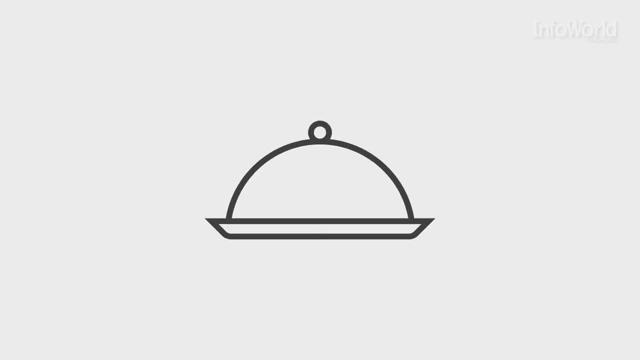 development teams do the same thing, giving each other feedback during the development work as well as at the end of each sprint in what is called a retrospective. At a restaurant, when a batch of orders is done, the next batch starts up following the same process. This 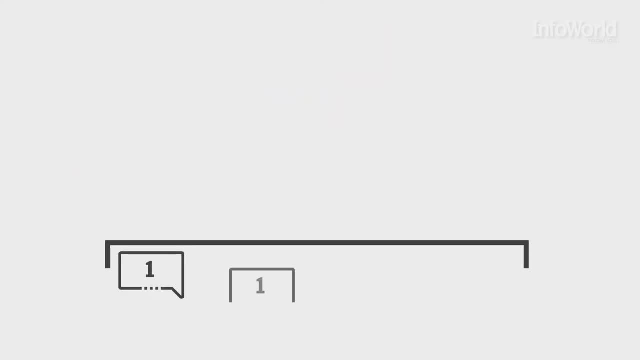 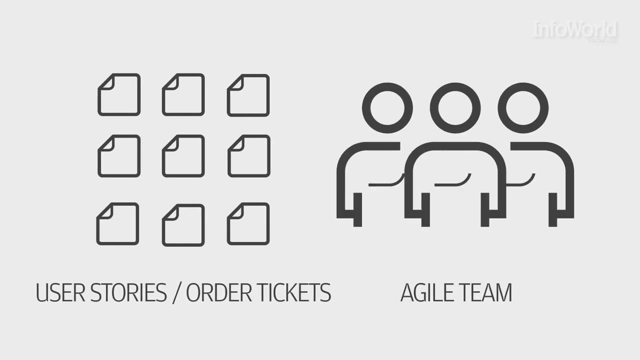 continues until service is completed. In agile development, the sprints continue until the product is delivered. When that happens, the team starts over again on a new product In a restaurant. the team will continue to work until the product is delivered. When that 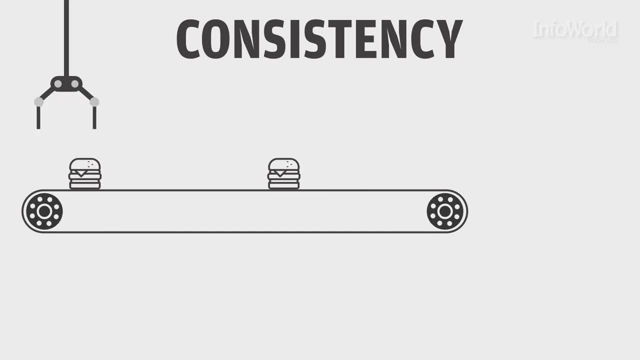 happens, the team will continue to work until the product is delivered. In a restaurant, consistency is important for every item on the menu. It's almost an assembly line for food. To accomplish that, the executive chef works out the recipes and then teaches them. 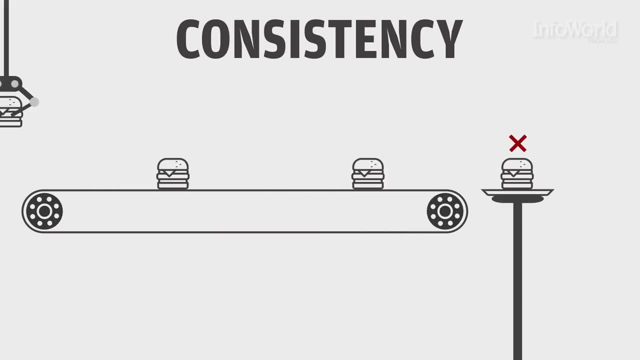 to the cooks and sous chefs. Typically, prep cooks also cut up all the vegetables and other ingredients in advance, to precise specifications, so they're ready to use when the cook needs them. In agile development, some of the work can be automated, such as code management.